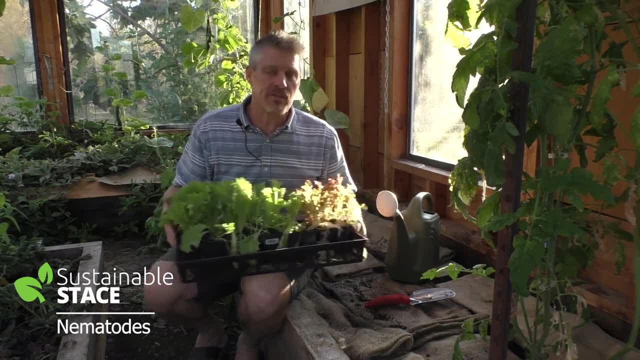 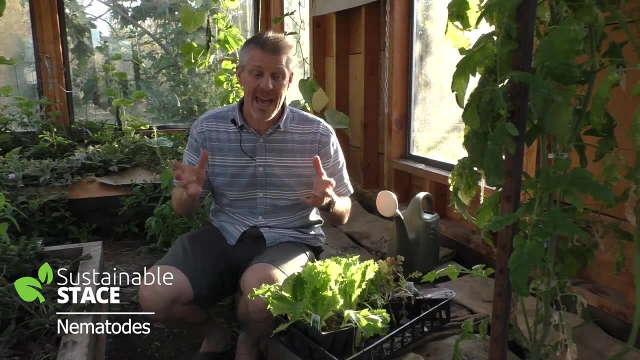 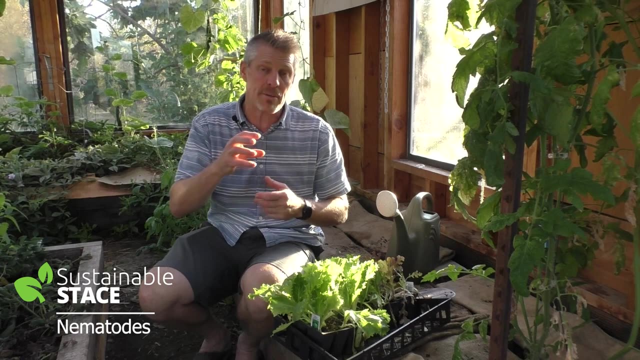 diverse, but there's a few specific strains of nematodes that are especially beneficial in your soil, because what they do is they take out several hundred types of pests that dwell in the soil in their pre-adult form, So something like a beetle might emerge in as an adult and come out and be. 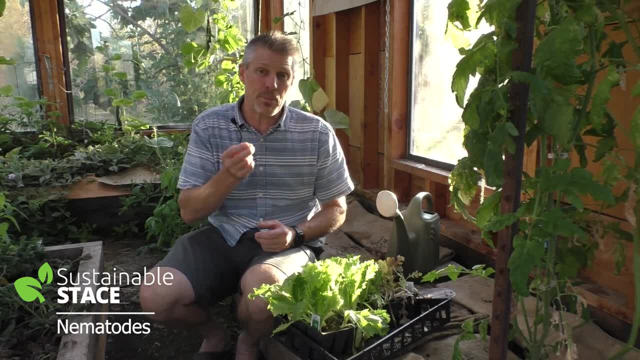 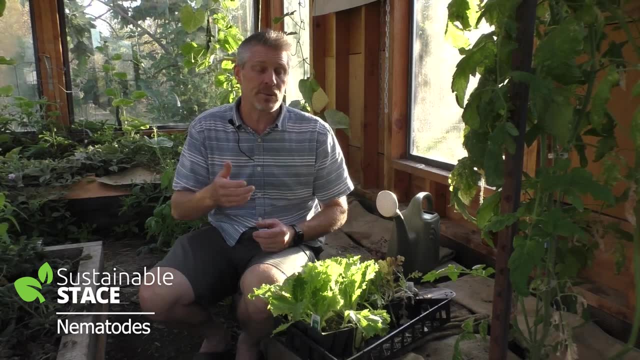 a problem in your garden, but a nematode can take out the pre-adult form of that beetle in the ground, in the soil, at the egg stage or at the larva stage. They'll do that with other types of things like weevils and borers as well. There's so many problems in our gardens that 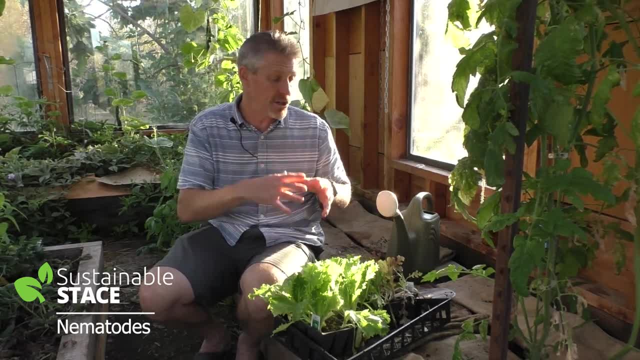 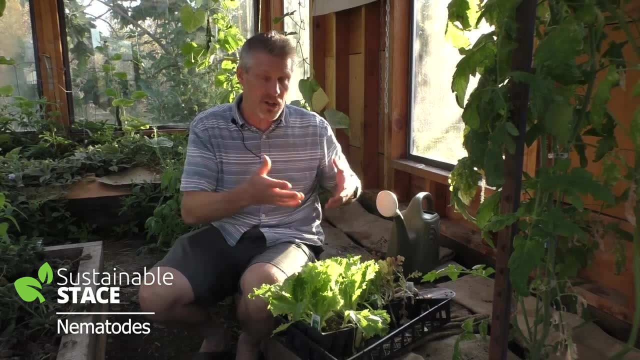 can be resolved with a good nematode level population in the soil. So that's why we're doing this today. I'm confident, certain, that with proper nematode application this lettuce is going to thrive where previously it was going to be toast. So with that knowledge and knowing, 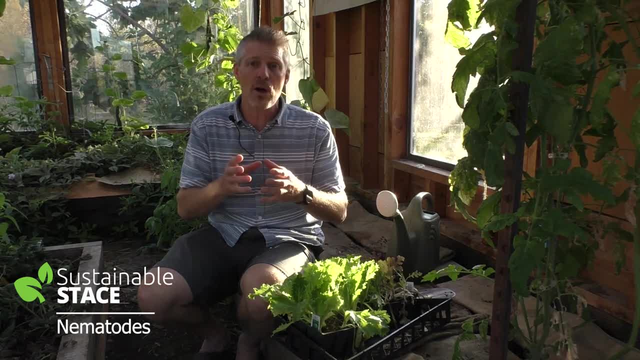 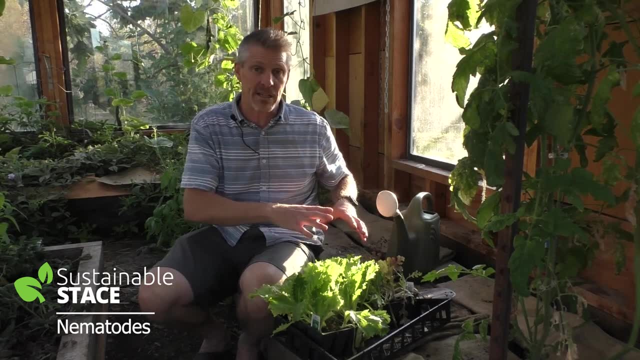 that nematodes- though you can't see them- are fighting for you. they're actually round worms that are microscopic. We're going to get to doing something that I normally never do. I'm always covering my soil to protect it, but I want to. 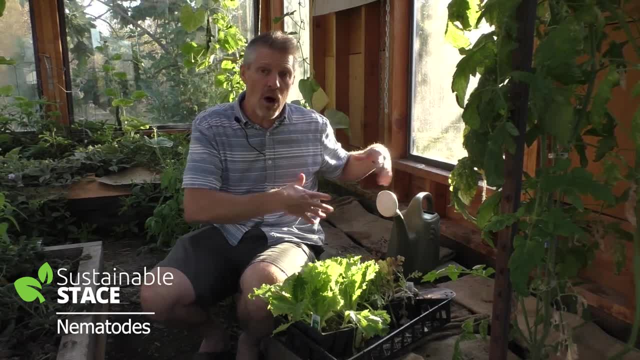 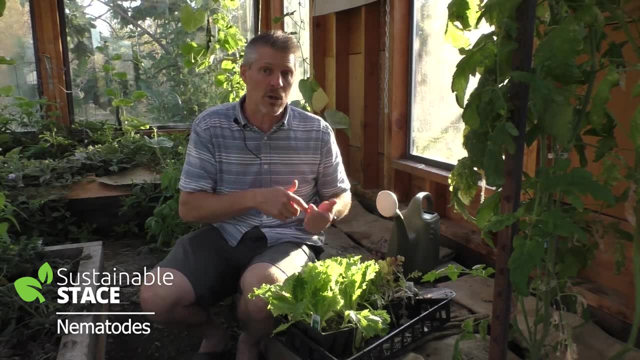 expose the soil before I sprinkle the nematodes all over it and water them in, because that's part of the instructions. watering intensively for three days, And I'm confident with that, we're going to see success in the soil where previously the lettuce didn't have a chance. So we'll just 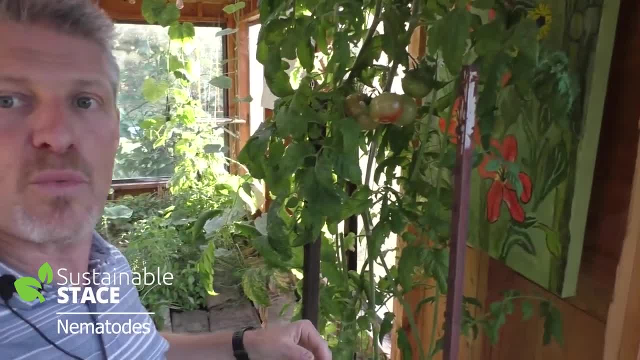 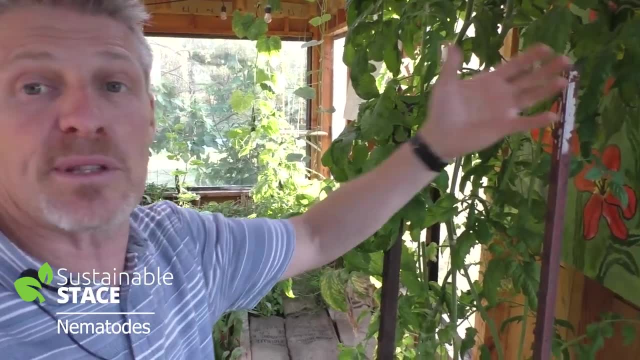 uncover and sprinkle and water and we're good to go. And while we're doing all this, you'll probably see that I'm always working around this one plant. that's kind of in the way, And the reason is it's October in the grow house and outside all the tomatoes have died. 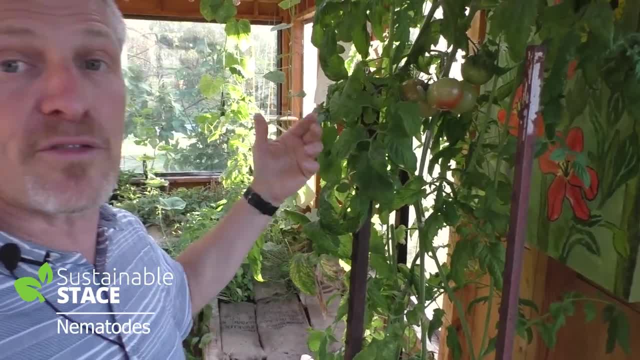 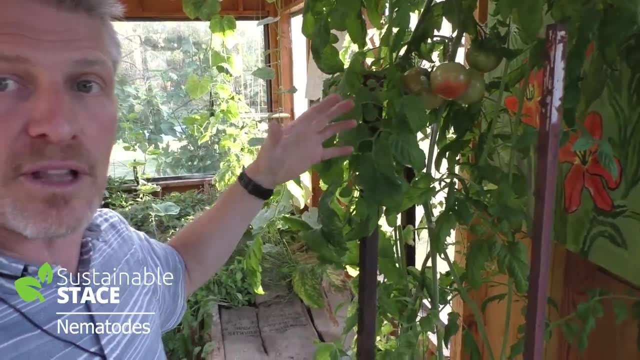 already. But here in the grow house I've got so many still ripening in different parts, But on this side of the grow house just this one plant remains, and it's got four big beauties on it still. So I'm wanting them to live out their life. while I work at the soil level to move the sacks and get ready, 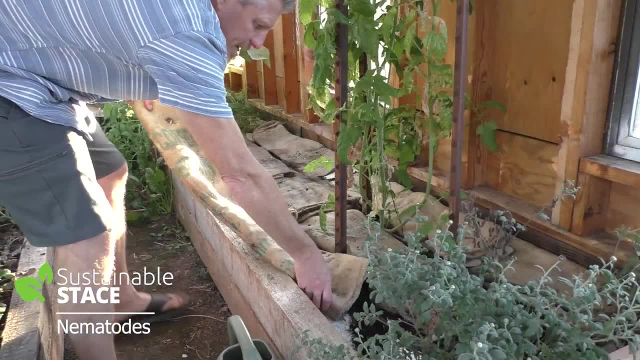 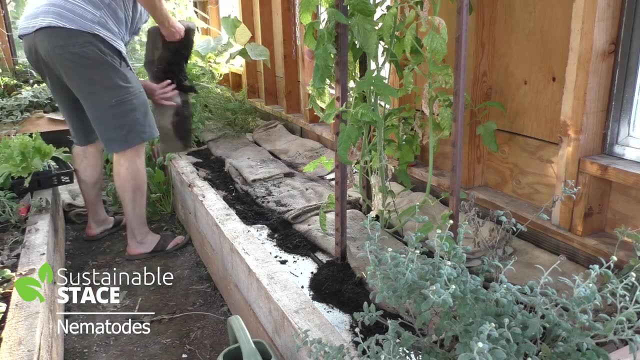 to plant the lettuce all around the tomatoes. Here we go. Yes, I'm going to remove all of the covering. One of the reasons is that I know I've got another enemy of many of my baby plants in here, And it's wood bugs. The wood bugs are all over in my soil. Have you guys seen wood bugs? 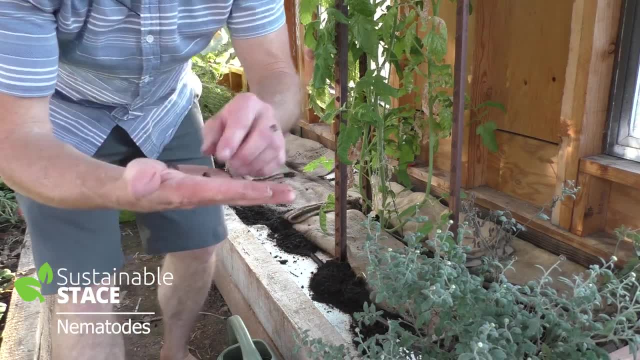 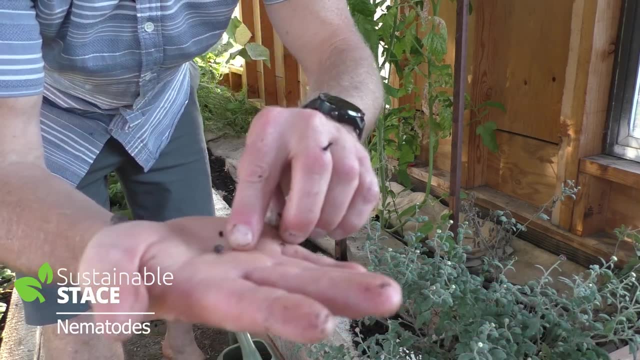 before. As I uncover them, they curl up. Here's a big one and a little one. You can see them crawling around here And when they're deciding to hide, they kind of turtle and curl into a ball. This one here has curled into a ball, but it's actually a wood bug. Same as that, It's just. 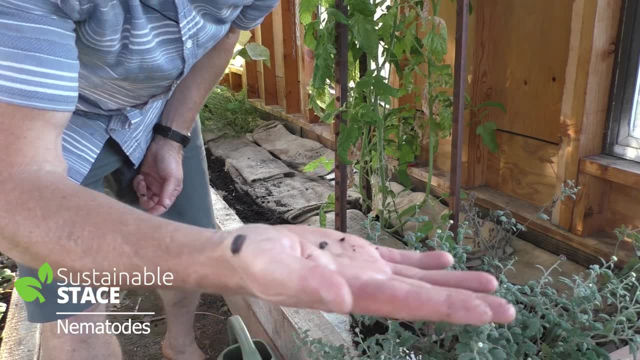 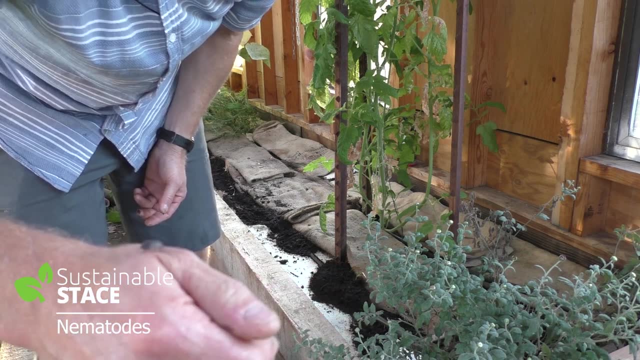 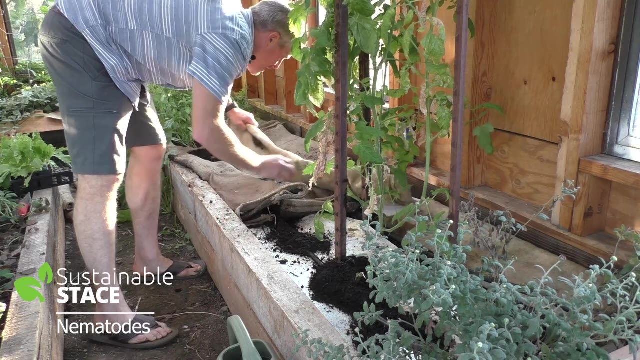 decided to hide And they eat all sorts of infant plants in my grow house if I don't uncover the soil, And then they scurry and hide just like a cockroach for shade. So they're a bit of a problem. So, continuing on, I'm just going to uncover all my soil. The worms are going to head. 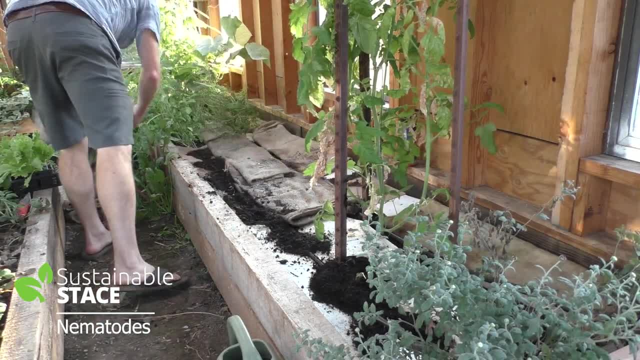 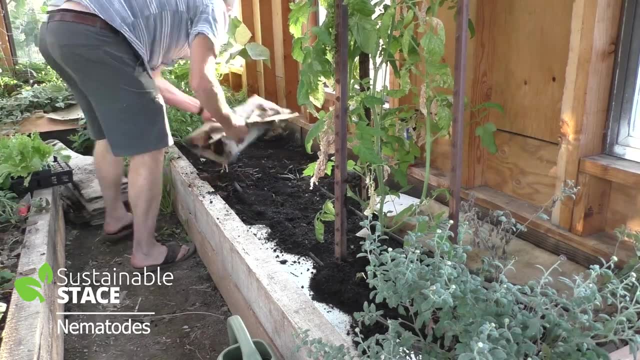 under right away, because right now they're at the surface And I see them diving right away And with this uncovered, we're going to be ready to go. This is a variety of nematodes, by the way, called Steiner Nema, So it's a Steiner Nema. 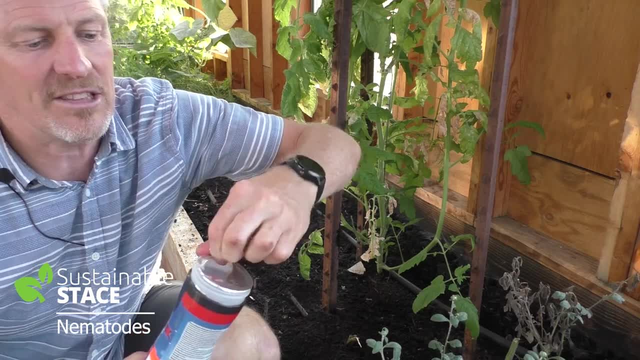 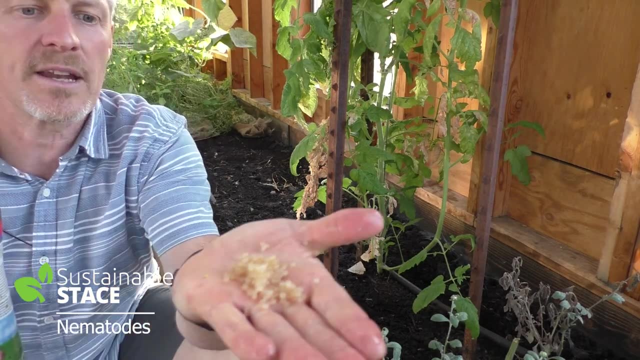 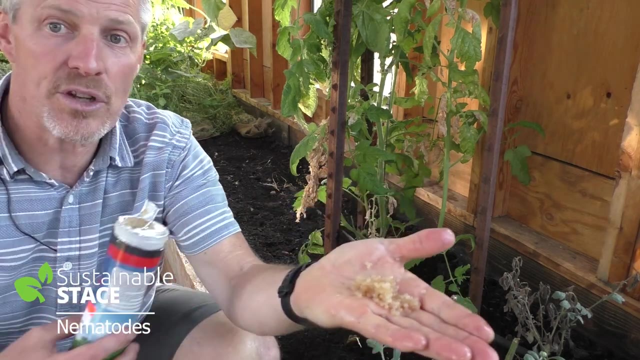 variety of nematodes. I've just broken the seal that's on the lid And I just want you to see what I'm seeing when I open them up. Do you see that Tiny little eggs that are going to hatch? The recommendation for use and distribution is spread it out over the top of the soil and water. 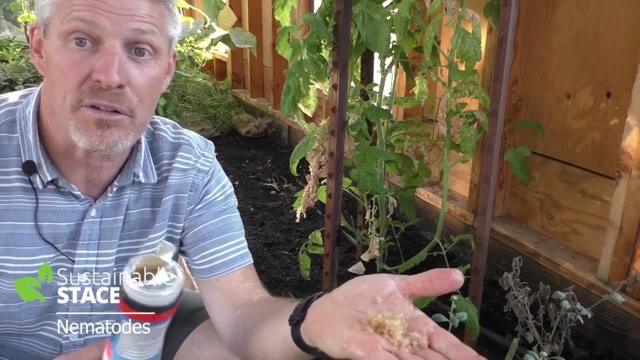 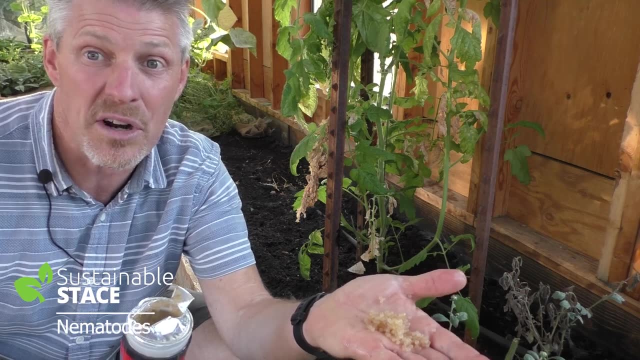 it in for three days straight And with that they will take off and their life cycle will restart. Currently they're in a state of what's called cryptobiosis. They can kind of suspend life when conditions aren't great. So we're pulling them out of cryptobiosis and sending them to war underground. 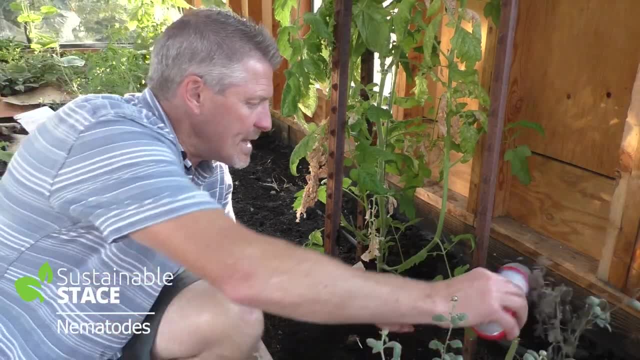 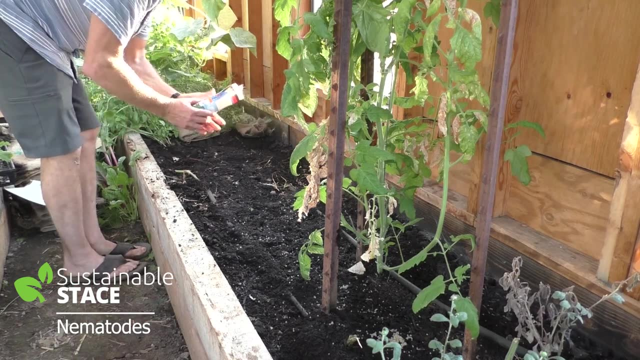 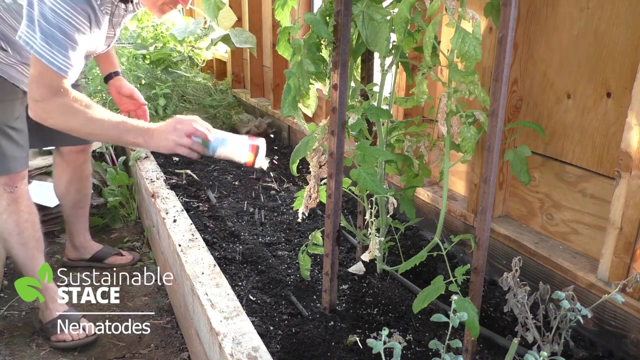 against the unseen. So we're just going to sprinkle them out, get them spread around all over, And with that we should be able to water them in and activate. Look at that, There we are, And with that, some water, And I'll do it again. 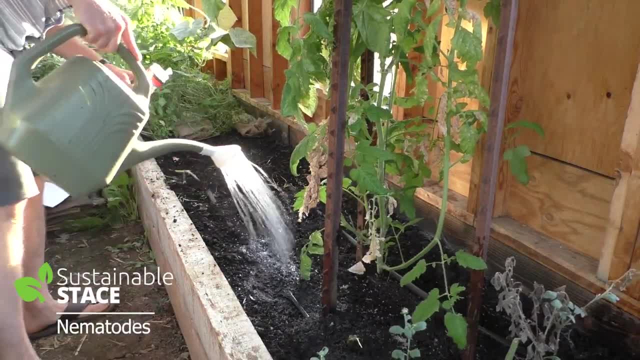 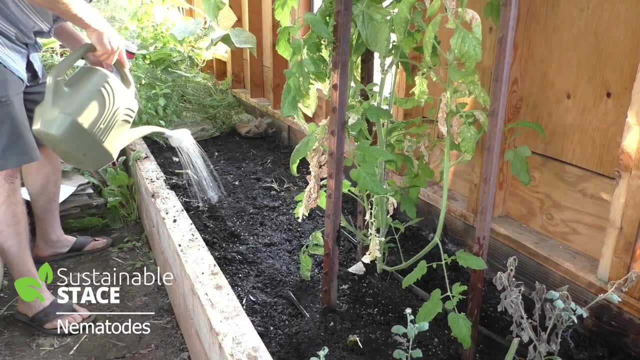 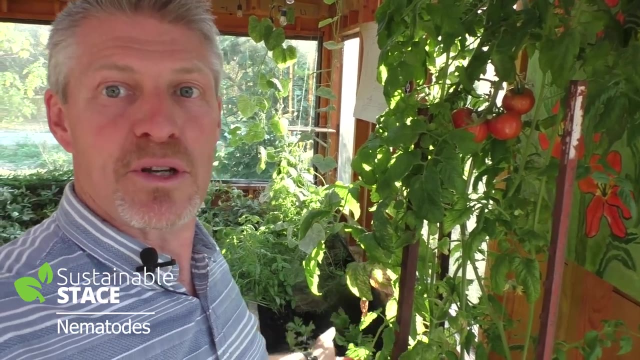 the next day And I'll do it again the next day, And those fellows are going to activate the Steiner. Nema Nematodes. Go, little guys. We get to win together. That's all there is to it. Well, remember guys that when we were getting the nematodes into the soil, I still had this tomato.